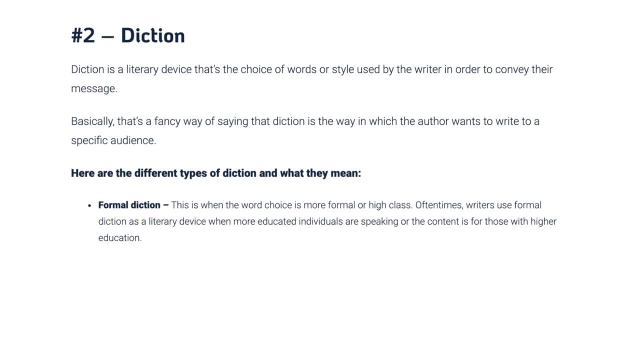 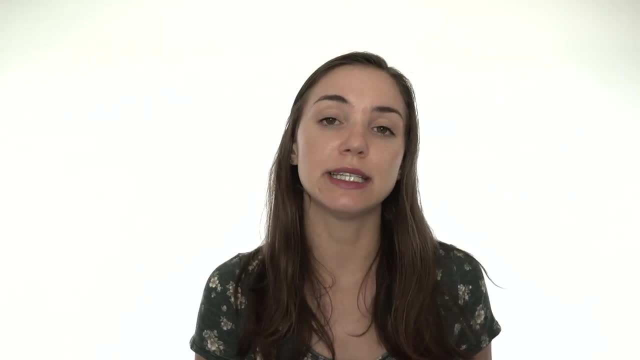 overall, We have formal diction, and formal diction is just, basically, when you're using more of a formal or a higher class, a more educated way of speaking. The reason you would use formal diction is perhaps when you have a book that is meant for more educated audience or you have a character. 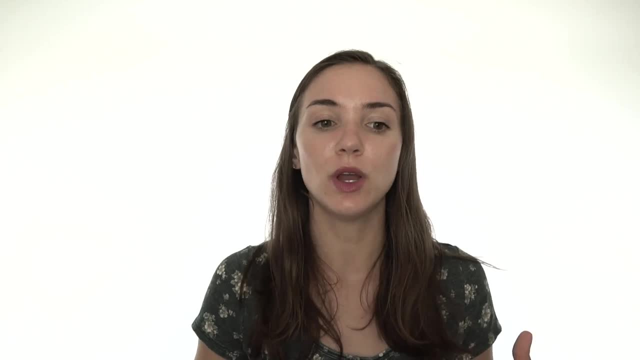 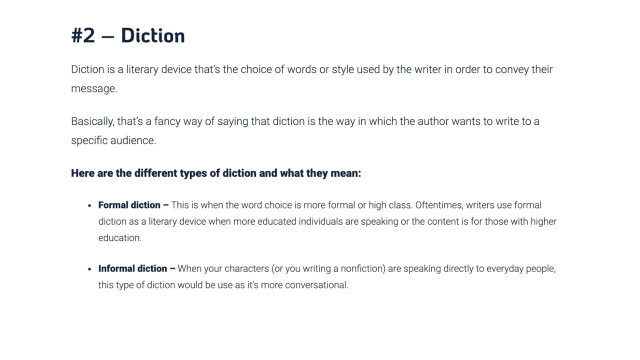 within your book who is of a higher class and you're hoping to share that message across. The second form is informal diction, and that's basically when your characters or you, if you're writing a non-fiction book- are speaking directly to everyday people. It's very informal. there's. 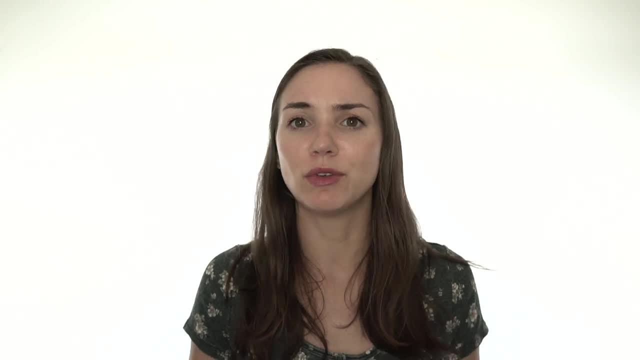 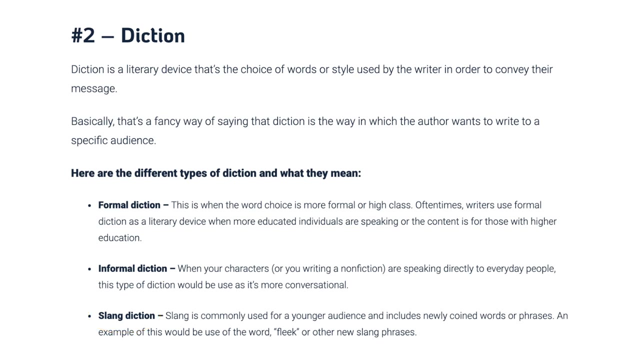 slang. there's a whole bunch of different things thrown in there. that is just a relaxed, formal, natural way of speaking. Slang diction is when you're using newly coined words or phrases or slang in your world. Now this can be real life slang, or you can make up slang for your own. A. 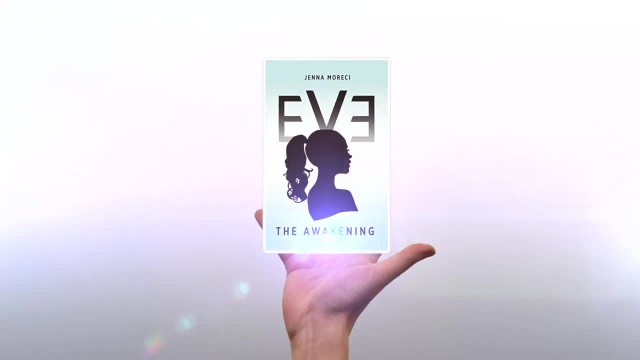 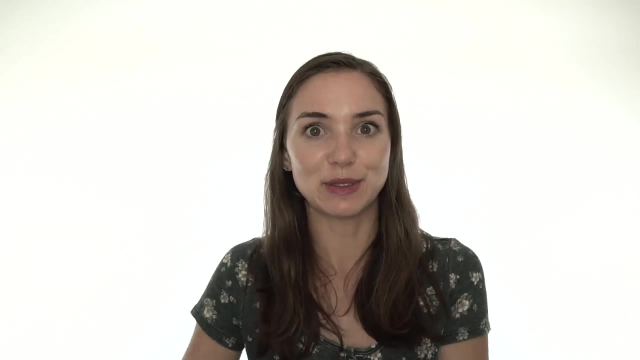 great example of this is Jenna Moreci does in her book Eve the Awakening. It's set about 80 years in the future and she created slang for her characters, because as we, as time goes by, we do create our own slang. so that makes it more realistic as well as just adding to that style of diction. The last: 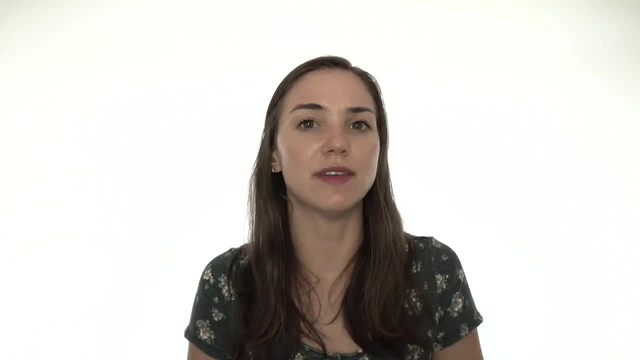 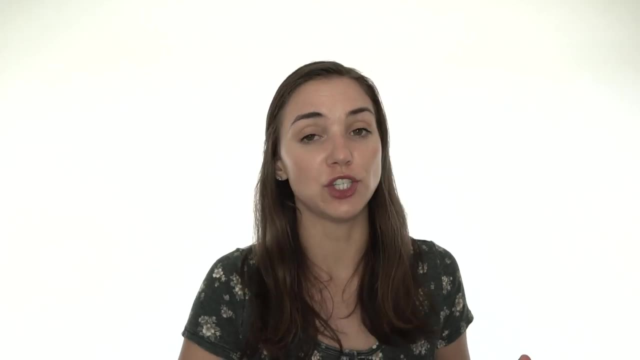 form is colloquial diction, which is basically just the use of everyday language. Now this might change depending on what culture and customs are In your novel, but overall diction is just the way in which you write the story, the book or certain people's point of views, if you have multiple in your book. An example of more formal: 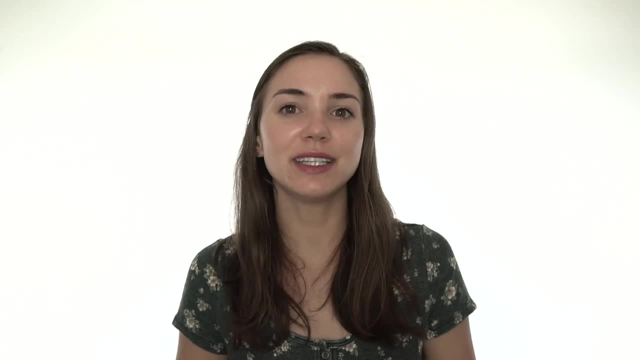 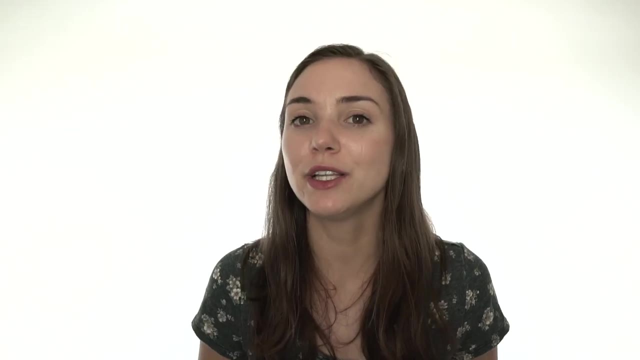 diction would be something like the phrase: I bid you adieu. It's not really something that you just say when you're saying bye to your friends, unless you guys have sort of a weird thing going on, but normally you'd say, all right, I'll see you later. That's more of an informal diction, whereas I bid. 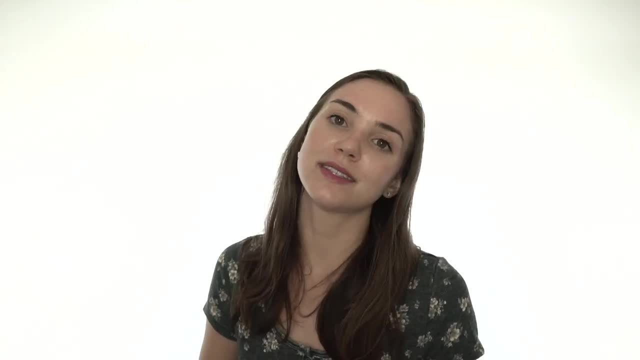 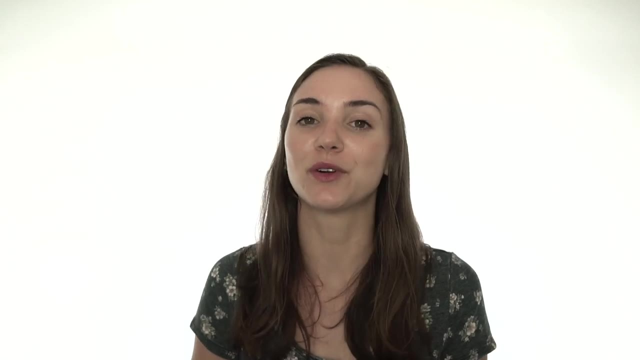 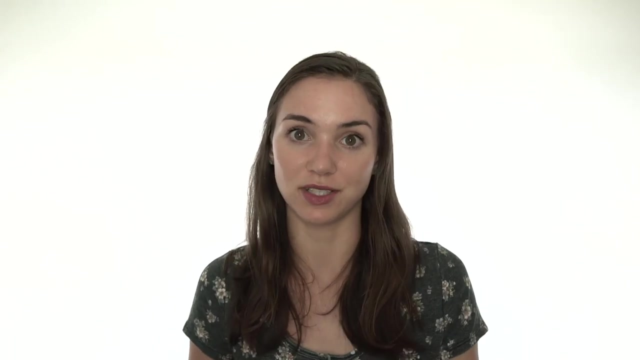 you. adieu is much more formal and proper. Another form is a sentence of: I remember her hair. it was like now. this is definitely more slang and informal. we're throwing in more of a recent slang word in general and it gives a much different vibe than the first example, and you can. 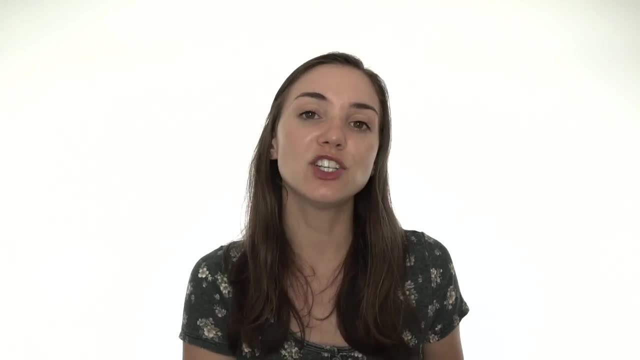 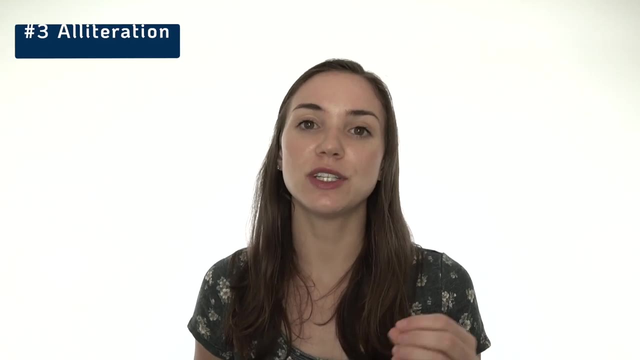 see that. so if you kind of focus on one throughout your whole book, it can change the entire tone and perception of what your readers are reading. Literary device number three is alliteration. Now, alliteration is basically the use of similar consonants right after each other in order to kind. 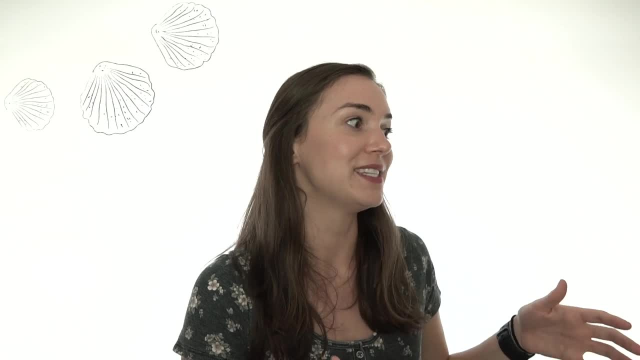 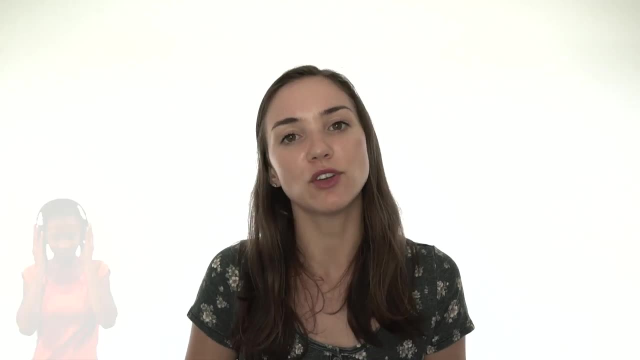 of make something sound the same. So a common example is: Sally sells seashells by the seashore. Obviously that's a little bit of a tongue twister, but alliteration is kind of used in order to give your writing more of a rhythm. This is probably more commonly. 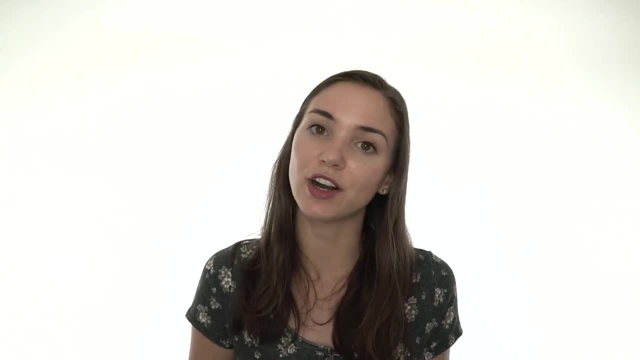 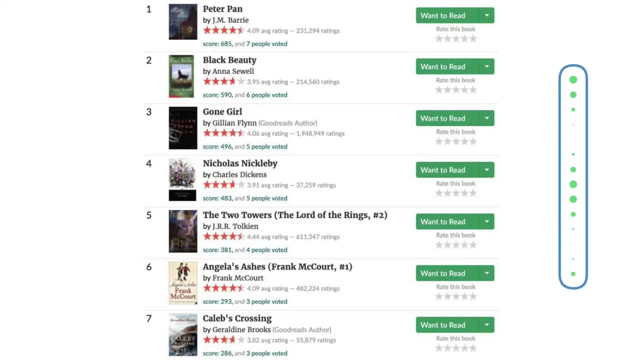 uh, seen in titles and in poetry. however, if you do bring this literary device into your writing, it can create something really special for your reader, something that has rhythm, even though it is just a novel or a book. A great way to use alliteration in your writing is to 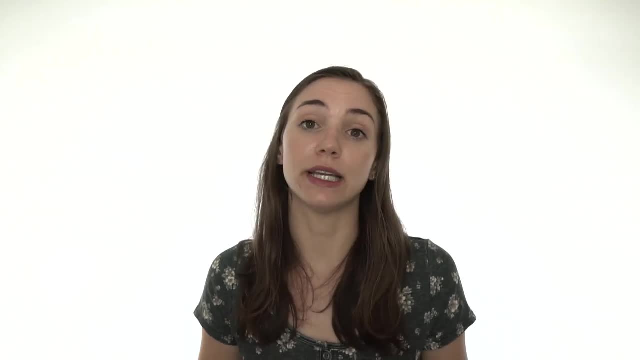 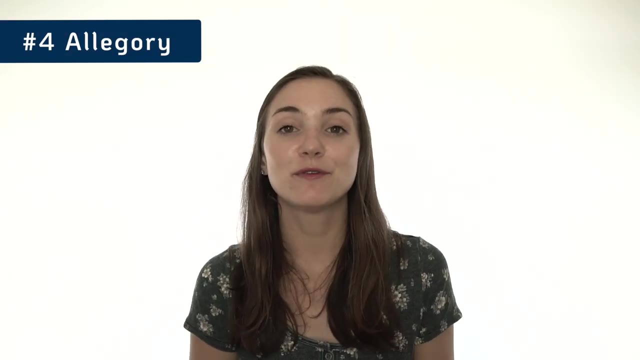 break up a paragraph that might be a little bit longer or boring, like a description in use alliteration in a few sentences in order to create a rhythm that is a little bit more exciting for the reader. Literary device number four is allegory. An allegory is a figure of speech where 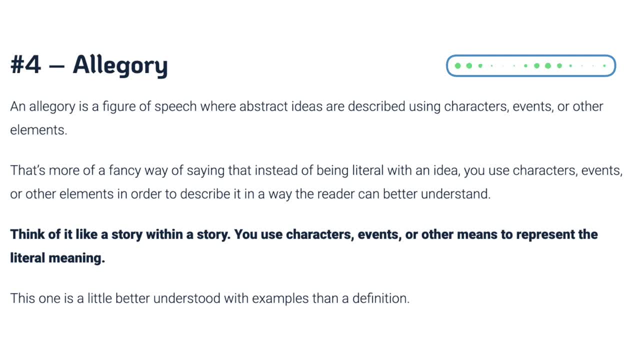 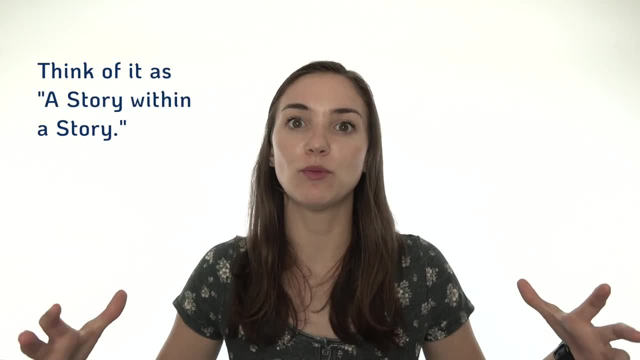 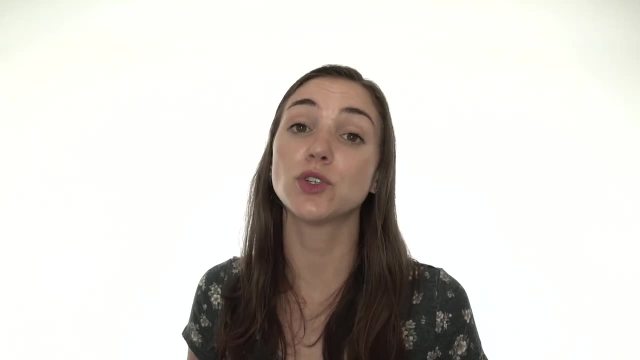 abstract ideas are basically described using events, characters or other elements. Think of it as a story within your story. It's as if you're telling a much bigger, more powerful message through a smaller, more digestible story. One of the most famous examples of this is in George. 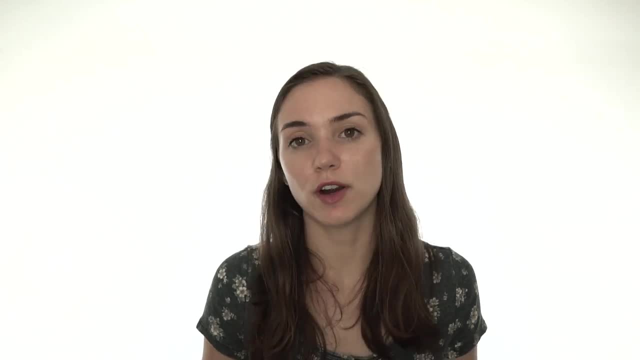 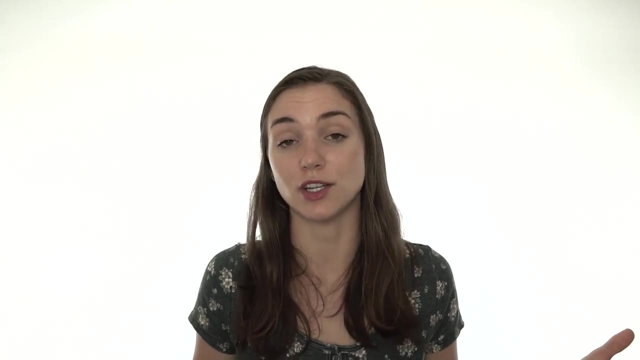 Orwell's Animal Farm. Basically, what the story is is where a group of farm animals basically kind of band together and rise above the um farm keepers, the, the people who are essentially in charge of them. Now that must might seem like a kind of a really inspiring little story, but what it's kind of based around 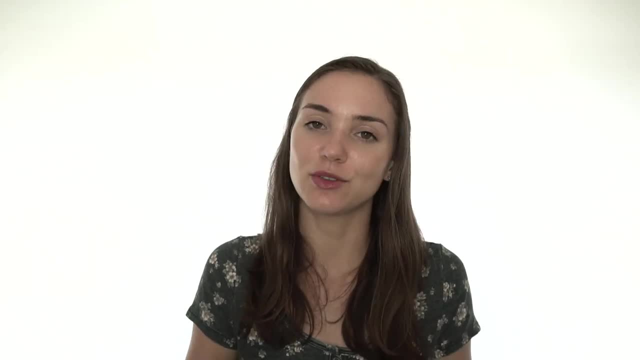 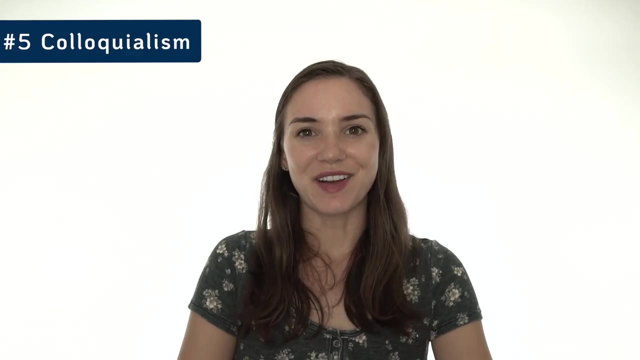 and what it's trying to tell the story of is the Russian Revolution, And so that's kind of. the example of the animal farm story is an allegory for the Russian Revolution. Literary device number five: colloquialism. Colloquialisms are expression, words and phrases that are used in 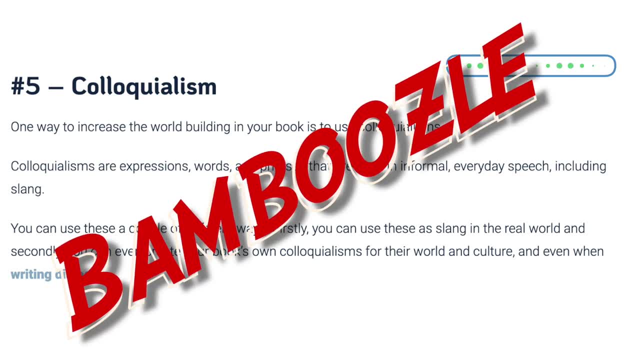 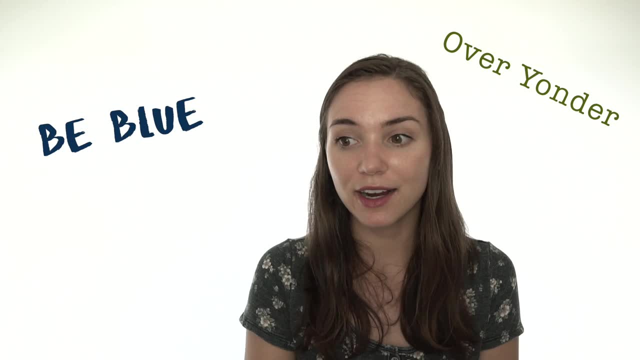 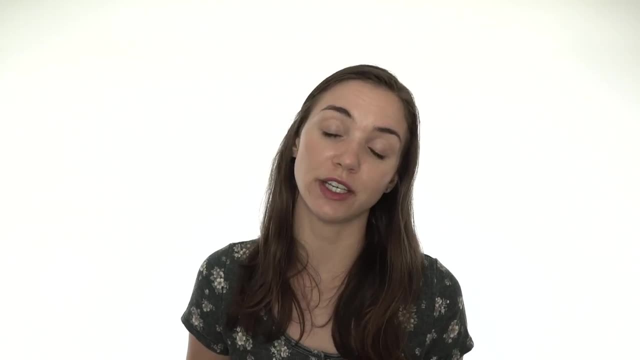 everyday speech. So a couple examples of this would be bamboozle or gonna um be blue as a way of saying sad Over yonder, to say over there Da bum, meaning the best. These are great to use just to kind of again set the tone for the novel or that character in particular. Connect your readers. 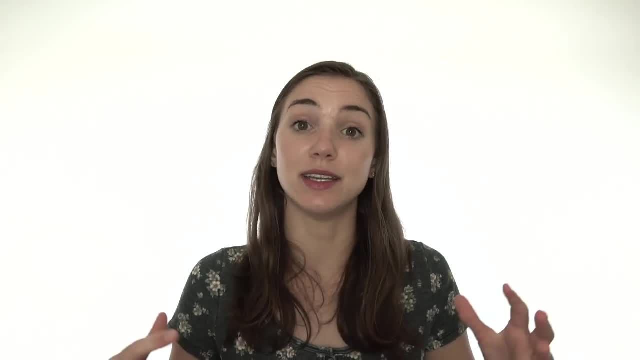 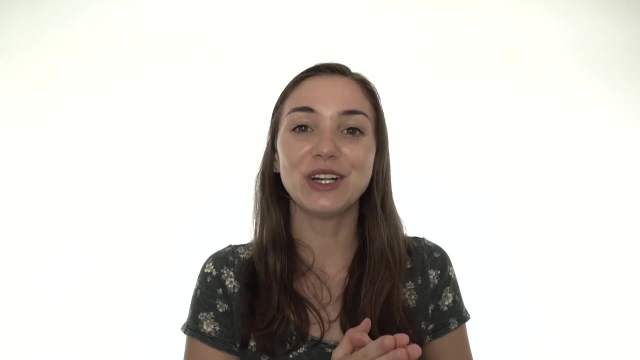 to the world a little bit more and if you're creating a story that's in its own world, you can actually create these different cool colloquialisms. Say that word five times fast In your own world. that can um help the world building a lot more Literary device number six is 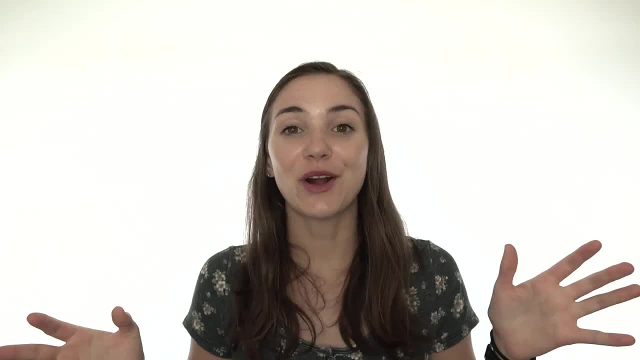 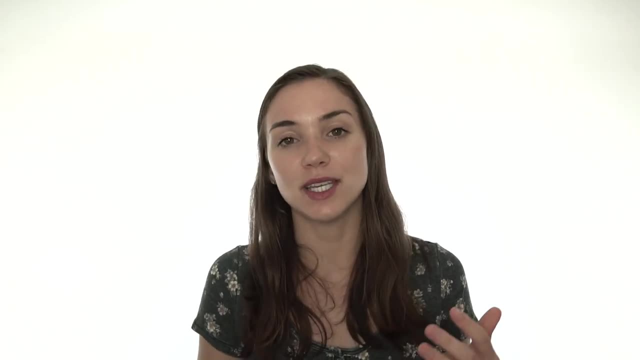 euphemism, and there are different ways you can think of euphemisms. There are different types of euphemisms, but one that probably popped in your mind right away are sexual euphemisms, probably just because they are ones that we use most often. But euphemism is basically just a kinder better. 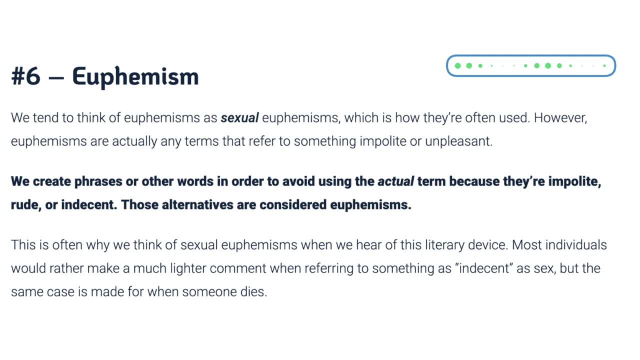 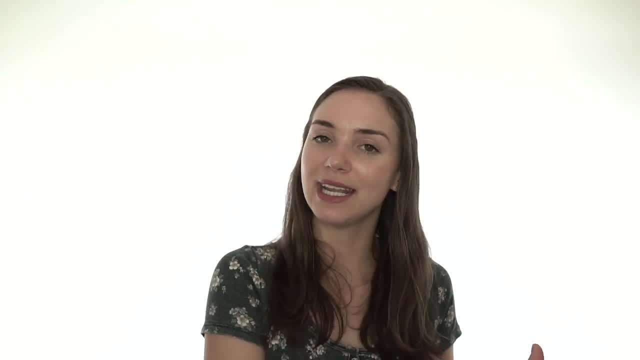 way of saying something that's a little bit harsh or distasteful or not appropriate for the moment, Which is often why sexual euphemisms get put into play. A couple examples of something that's not quite in that way but is still a euphemism could be saying: before I go, as in before I die. 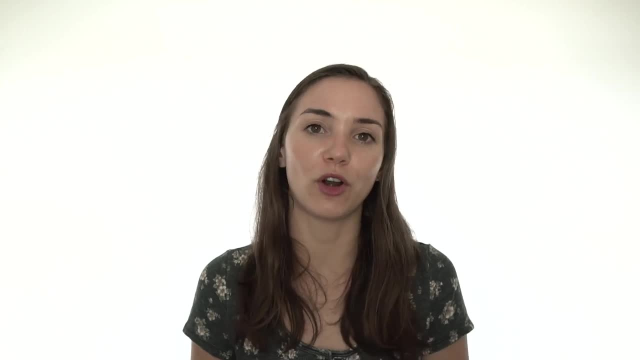 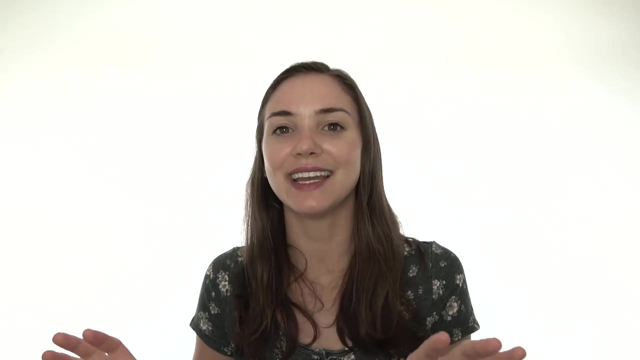 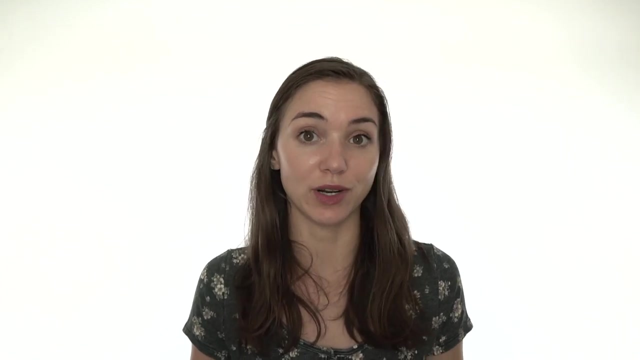 Or saying something like a rear end instead of butt, Or perspiring instead of sweating, Tipsy instead of drunk, Thin on top instead of bald, You get the idea Basically saying something a little bit nicer to avoid the harsher- even if it's more accurate- phrasing of what you want to say Again, 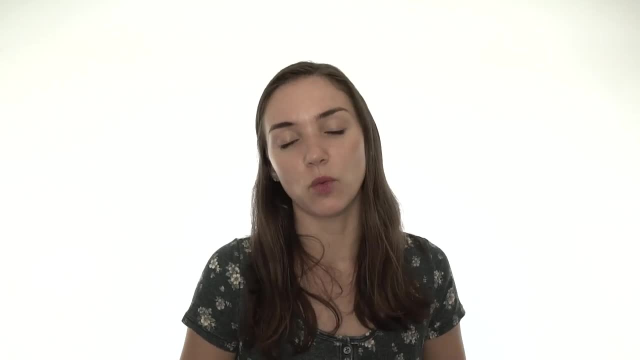 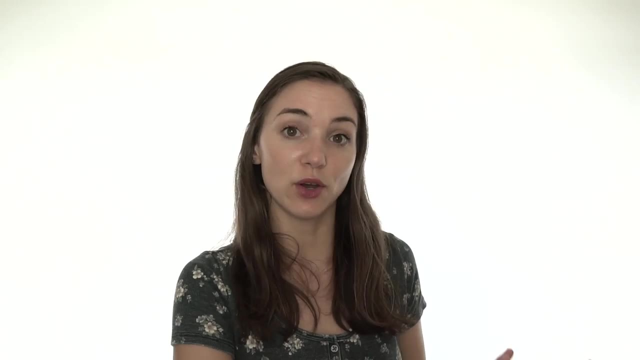 this is something that you can make up for your own world if it's set in a world that's not in her different customs and those different things might not be the same. So in my story I'm writing a fantasy novel set in its own world. there's a euphemism we say essentially they say you're. 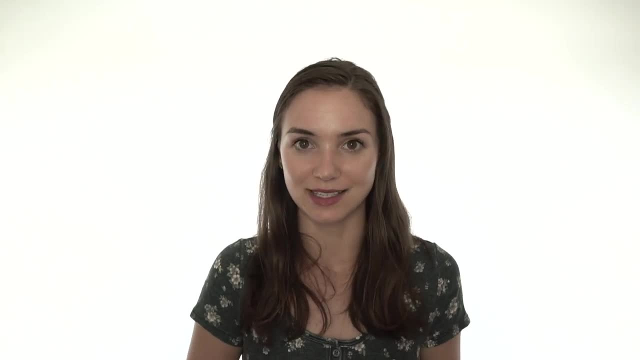 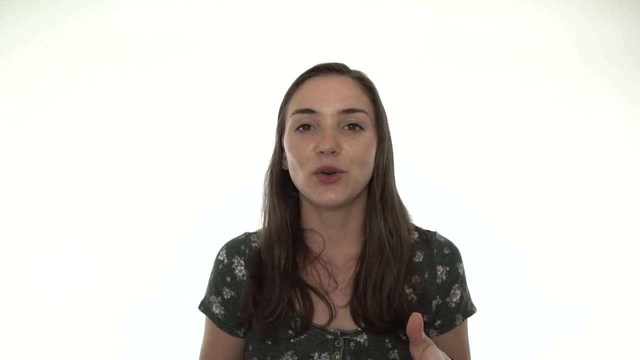 going to kill the tree And essentially what that basically means is that you're being lazy. So if you ask somebody, oh, are you just going to kill the tree, it's essentially saying: are you just going to be lazy and not do that? So these are types of things that you can create in your 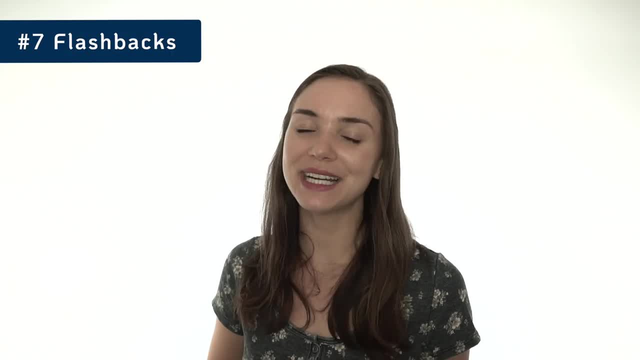 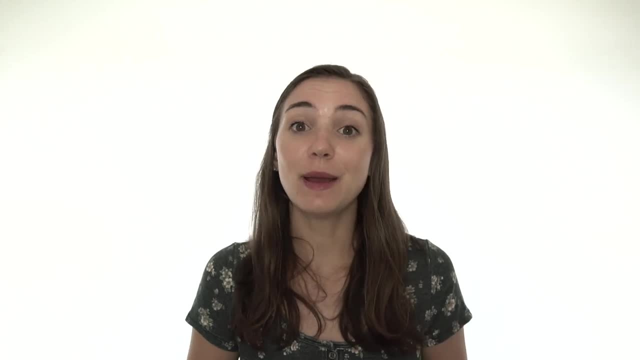 own world Literary device. number seven is flashbacks. Now we're getting into something that's a little bit more complex than it is just something that you can add into your writing. So flashbacks have to be very, very intentional, and if you don't know what a flashback is, it's just. 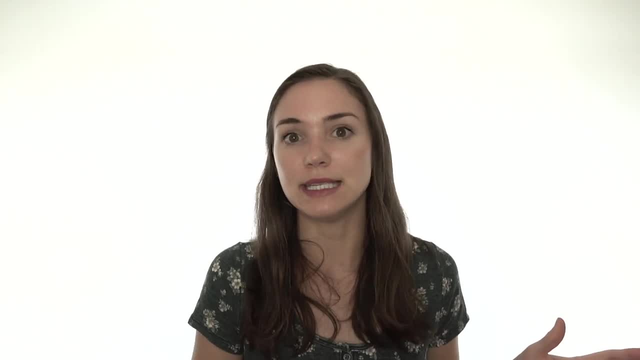 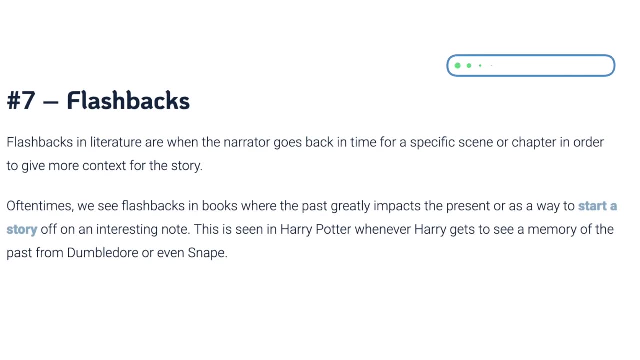 simply going back in time from the present place in your story or your book. Flashbacks can be used for a number of different reasons. It can be to further a plot point, it can be to uncover information the reader needs to know, or it can be used as a reoccurring plot device that either 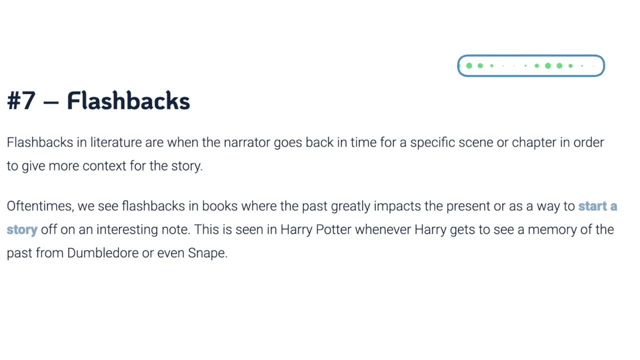 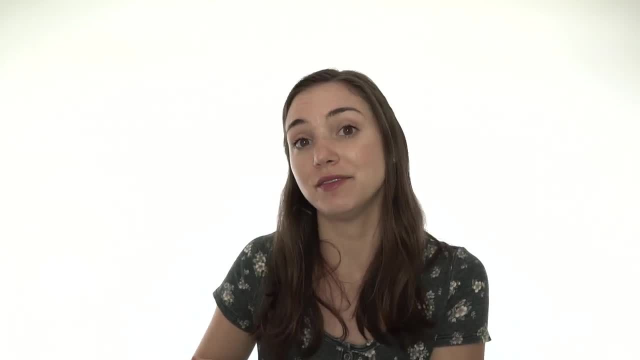 impacts your main character or helps them along in their journey. One book that does this really well is Vicious by VE Schwab. She uses the flashbacks as a literary device and as a plot device, So basically every other chapter she has. it goes back in time to some event and then back. 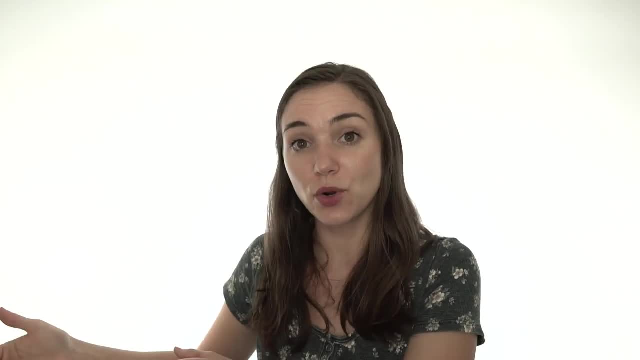 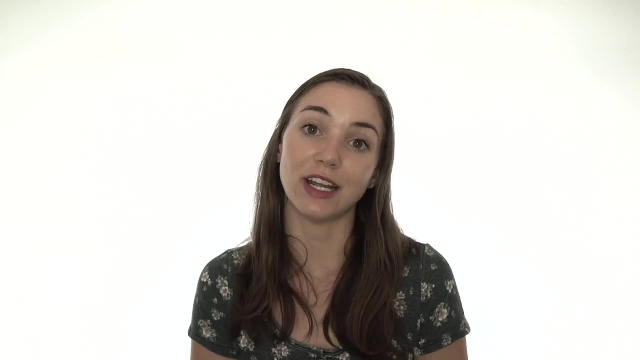 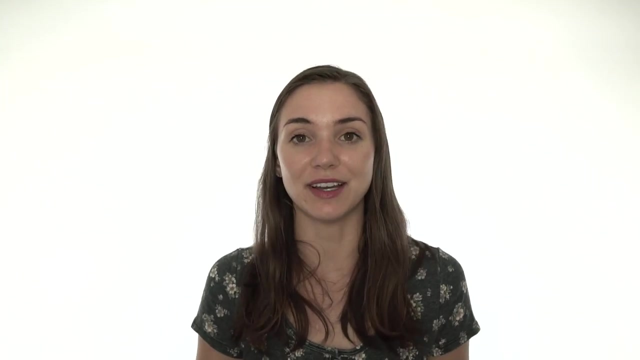 to the present, And so this because it carries on throughout the story. it serves as a plot device, and the one thing that you want to make sure with flashbacks are that they are useful and important. So if you want to get a good feel of how to do flashbacks in the present moment effectively, 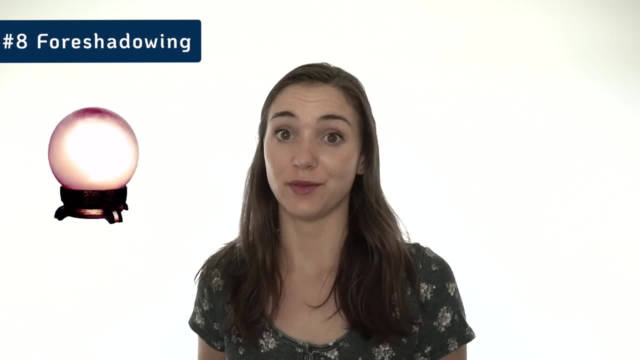 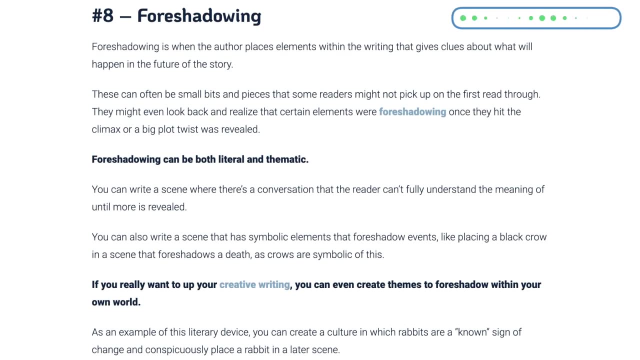 definitely recommend reading that book. Literary device number eight is foreshadowing. So foreshadowing- for those of you who don't know- is essentially giving hints and clues about what's to come in your novel. Essentially, you don't want readers to be able to pick up on those, but you want them to look back at the novel and be like 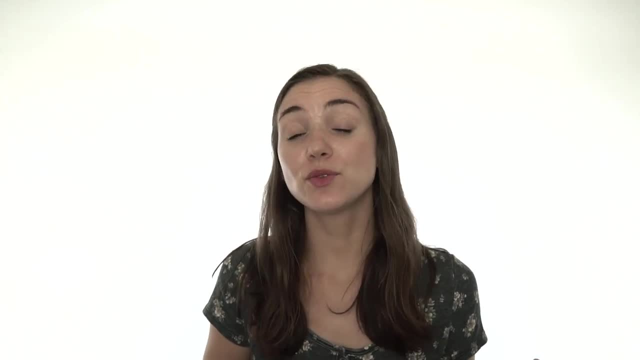 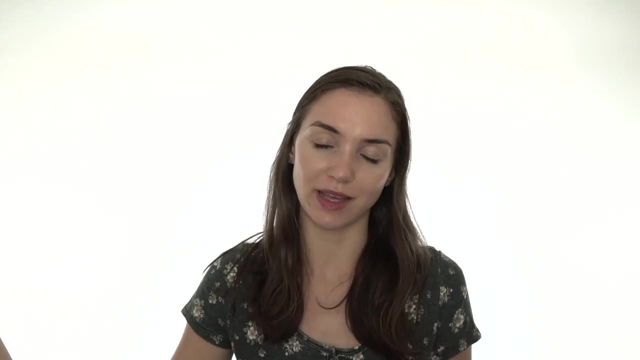 I should have known that I should have picked up on that detail. This is a really important part in your story because if you never give your readers any clues as to what's to come, they're going to be very confused by the outcome. But if you drop these little hints that they don't 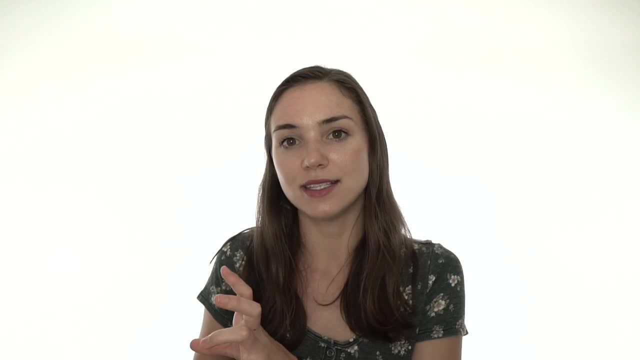 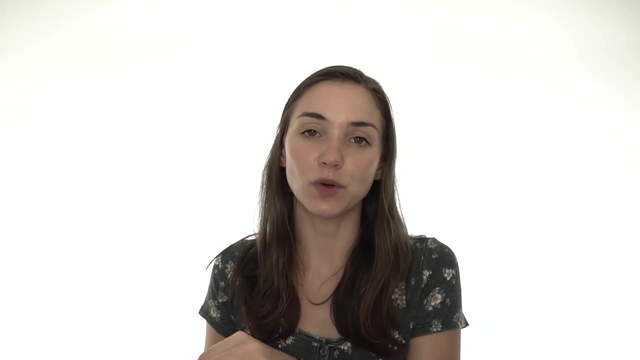 pick up along the way. but then they look back and they they realize, um, at the climax or whatever big event is happening that it makes complete sense and they should have seen it all along. that is what readers want. They want that surprise, but they want the surprise to make sense. 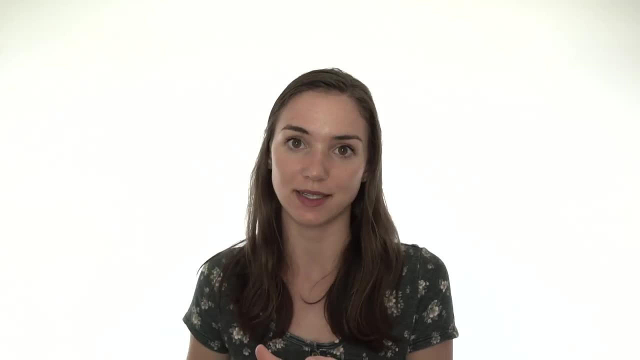 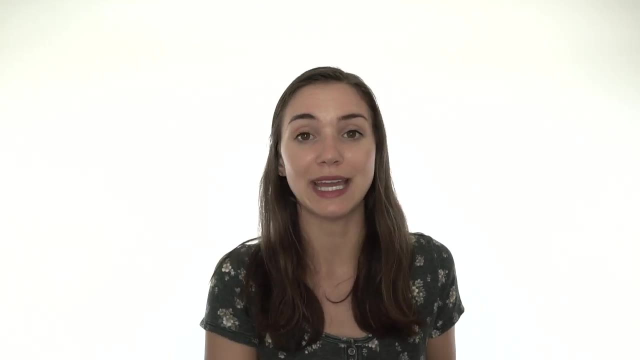 and the foreshadowing is how that surprise or that twist makes sense in the end. A really popular example of this in a movie specifically is in the Avengers movie, when there is a ship's engineer playing a game on the little computer and the purpose of the game is actually to 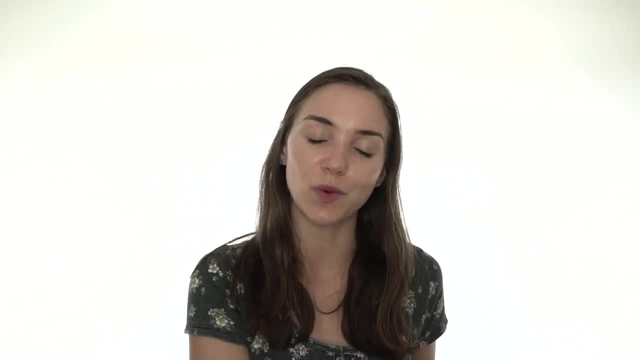 defend or defend the ship. So the ship's engineer is playing a game on the little computer and the purpose of the game is actually to defend or defend the ship- earth- from the alien invaders, which is what happens later in the novel. It's a very small. 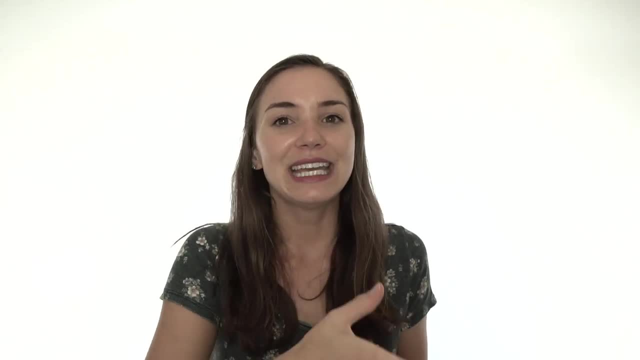 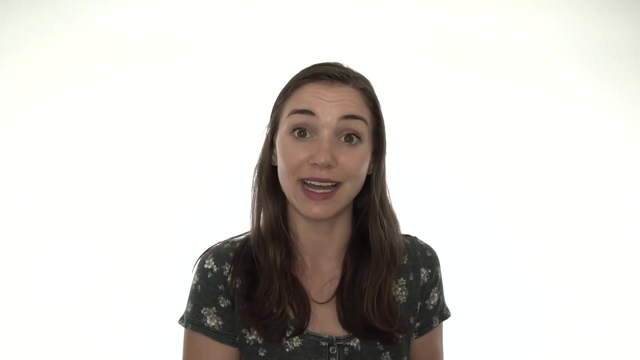 thing that very few people probably pick up on, but that even makes it just makes the end in the climax that much better. So if you can drop in those little hints that blindside your reader at the time, but then add up and make sense, in the end you will be doing foreshadowing effectively. 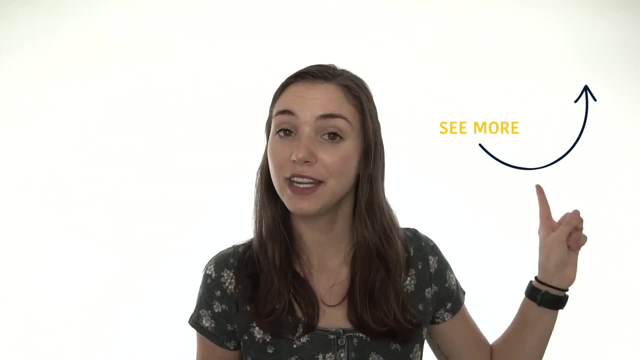 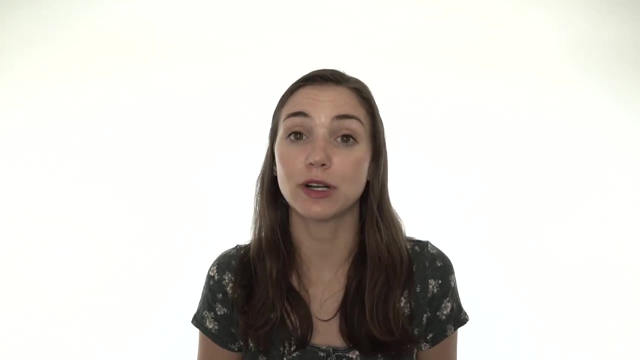 If you want more examples and want more tips on how to foreshadow, well, we have a video right up there for you to check out. Literary device number nine is imagery. Imagery is essentially use of visually descriptive or figurative language in your story in order to paint a much clearer 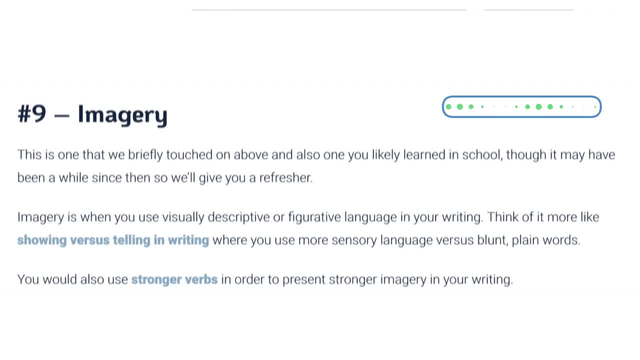 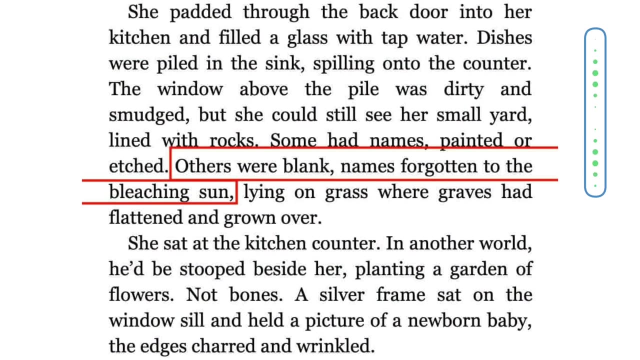 picture. Really. what you're trying to do with imagery, as the name suggests, is create an image in your reader's mind. There are several examples of this, but essentially, if you're describing something in detail and you're giving it enough description in order to paint a picture, you are 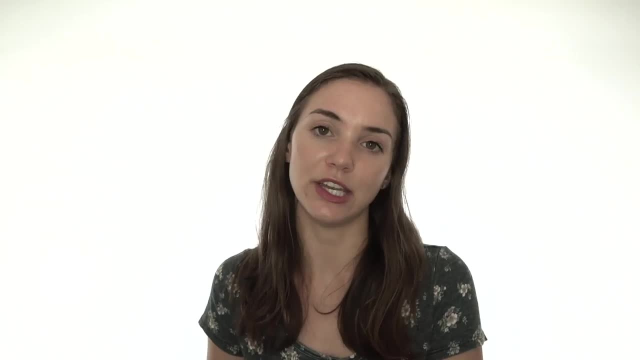 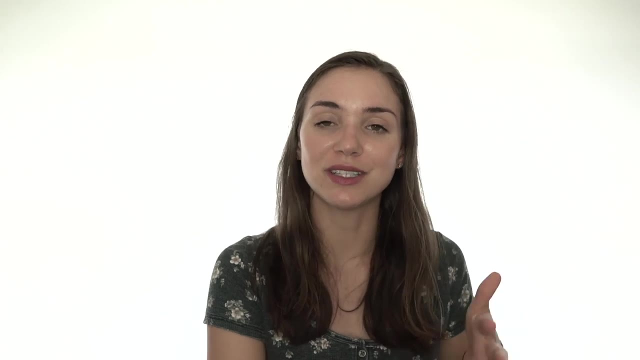 using imagery, and this also helps you show rather than tell in your writing as well. Literary device number 10 is personification. If you don't remember personification from middle school or elementary school, it's essentially giving human-like characteristics to non-human things. There are a 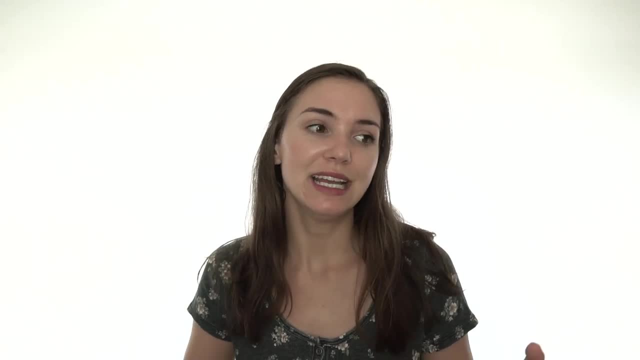 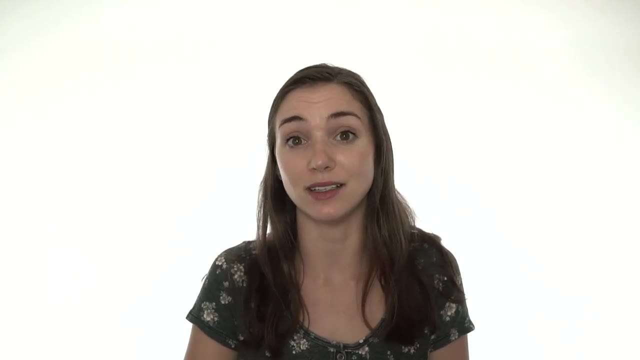 lot of really good reasons to use personification. One in particular is that it just brings a new element to your writing. It is a new perception and perspective that your readers probably don't get a lot, and it allows you to uniquely craft how they view different things. A couple of examples: 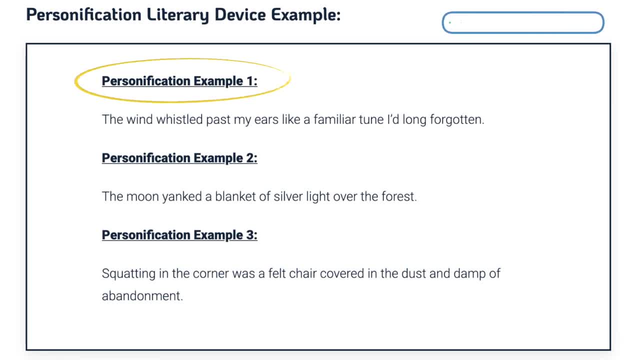 of this are one. the wind whistled past my ears like a familiar tune. I'd long forgotten The reason. technically we use that a lot, but it's technically a human trait. The second example is the moon yanked a blanket of silver light over the forest. So this essentially, is giving the moon the power. 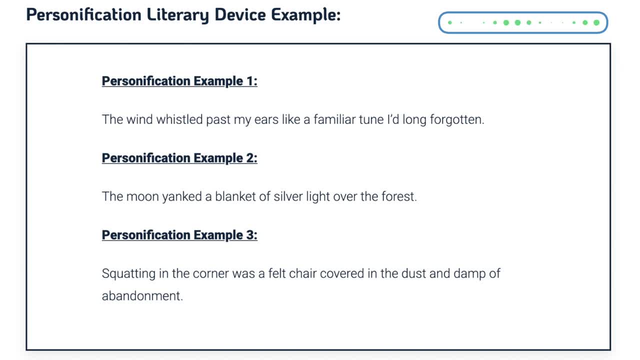 to yank a blanket up, kind of like, you know, a parent or such. Example number three is squatting in the corner with a felt chair covered in the dust and damp of abandonment, And so essentially we're giving the chair the human trait of being able to squat. So this just adds a little bit more. 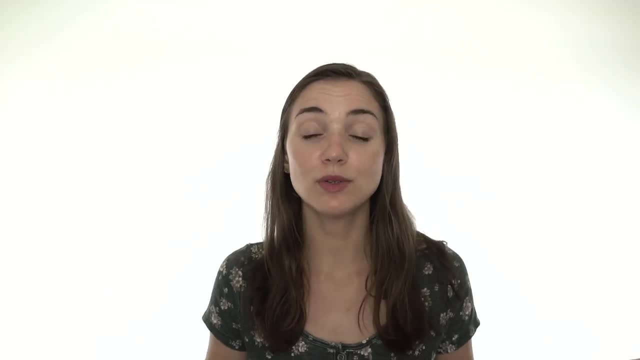 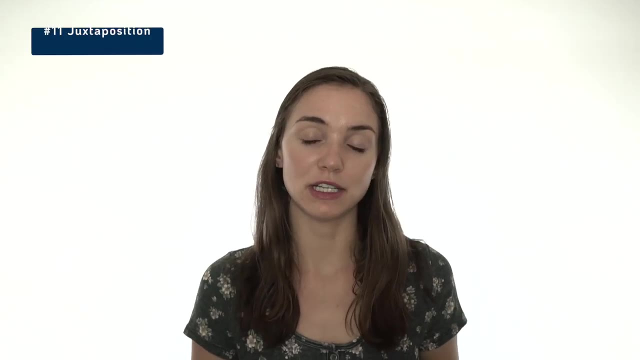 to your writing. It allows you to craft a little bit more of that human trait of being able to yank a blanket up, kind of like you know a parent or such. Example number four is juxtaposition. This is probably one of my favorites because it allows you to craft and kind of manipulate the 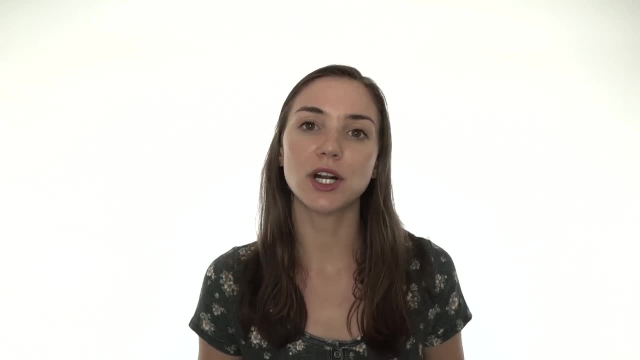 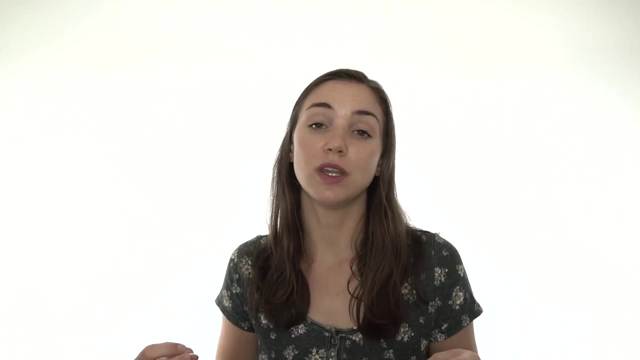 emotions of your readers, And juxtaposition is basically putting contrasting elements next to each other in order to amplify them a little bit more. There are a few different ways you can do this. You can actually do this within words themselves or sentences. You can do this with 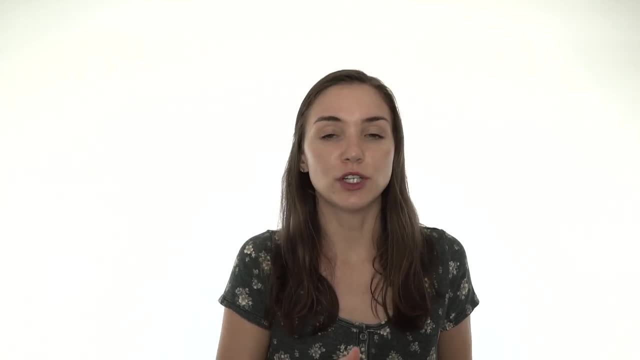 themes, and you can also do this within chapters. You can actually do this within words themselves or sentences. You can do this with themes, and you can also do this within chapters. So a big thing that I've learned, and what I find that I love the most in books, is when you 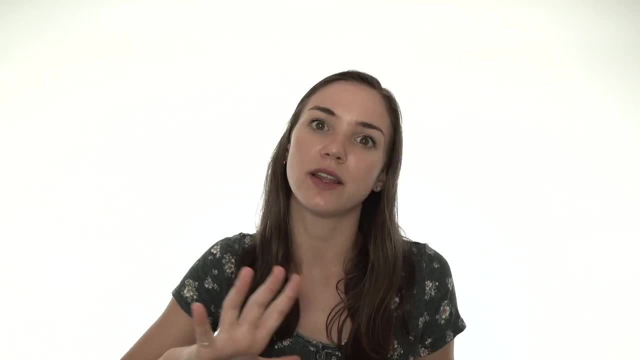 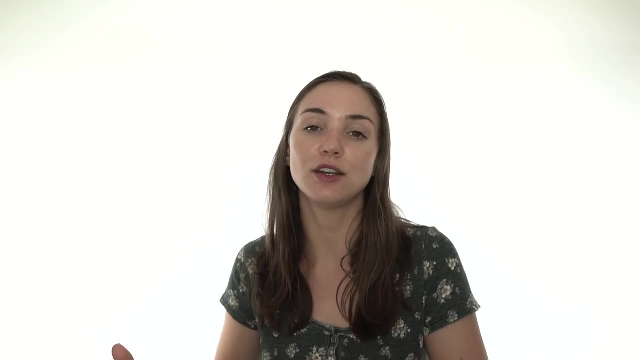 end a chapter on a sad note and then you start the next one on like a happy or a higher note. So that roller coaster of emotions effect that a lot of readers love is going to be done through juxtaposition, And here are just a few examples of that. So example one number one would be: 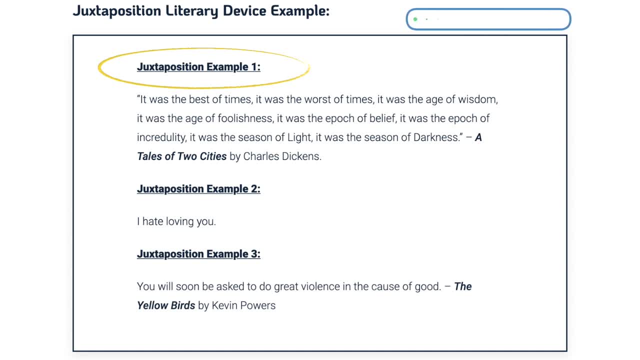 something along the lines of this famous phrase of it was the best of times, it was the worst of times, it was the age of wisdom, it was the age of foolishness, And so those contrasting elements right next to each other helps to amplify the message as a whole. 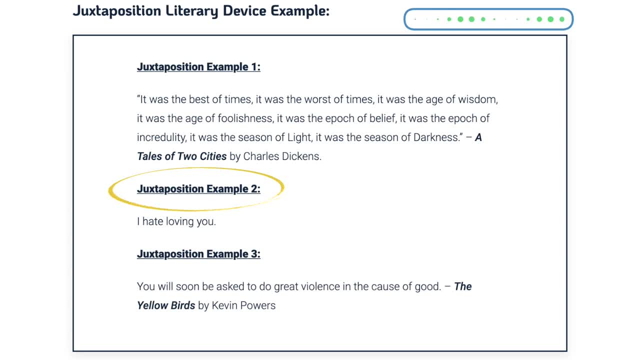 So example number two is: I hate loving you. Something that simple can really impact the emotion of what is being said and which character, or, if it's you and you're writing a nonfiction book, what that means to you. And so example number three is: you will soon be asked to do great violence. 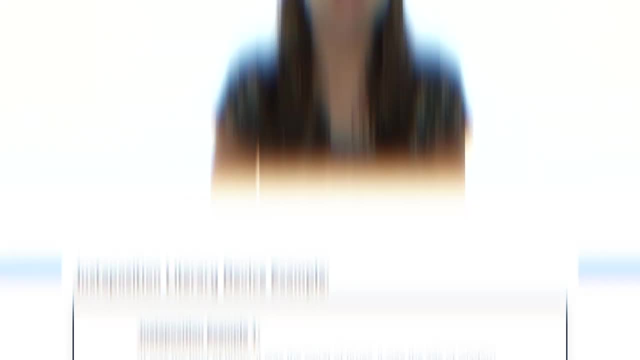 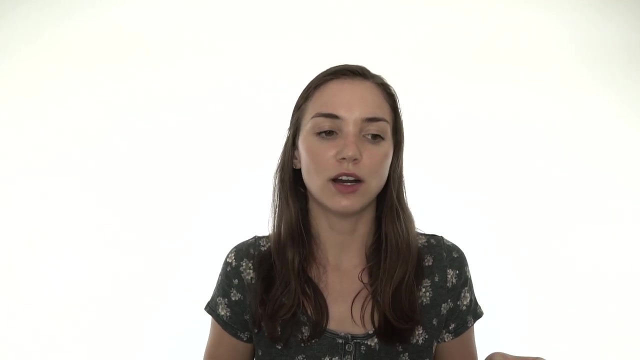 in the cause of good, And this is very important, because good and violence are very different, contrasting elements, And so, as you can see in these examples, what you get is something much more powerful, because you are placing those contrasting elements right next to each other. 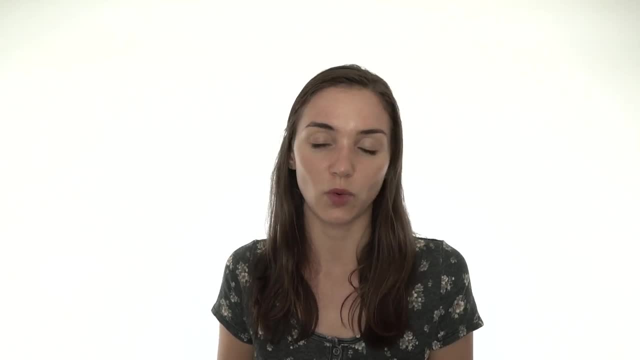 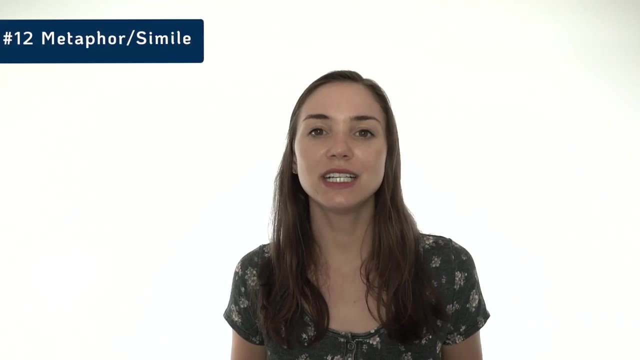 So don't think that you have to do this within just sentences or words. This is something you can do on a much broader scale, throughout the entirety of your novel, from scene to scene, chapter to chapter, etc. Literary device number 12 is a metaphor or simile. Yes, I know they're. 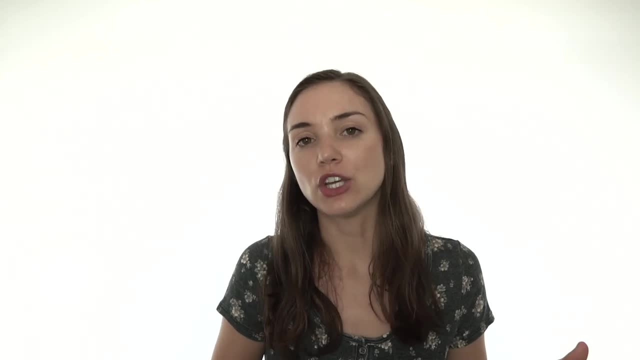 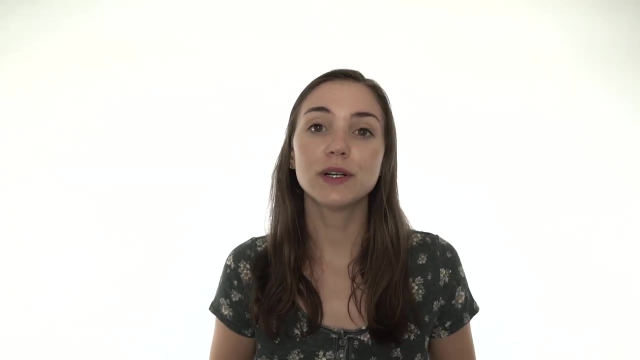 different, but they are very similar, so we're lumping them in one. Metaphors and similes are basically comparisons used in order to help your reader picture something better or understand something a little bit better. A metaphor is basically things that are not alike being. 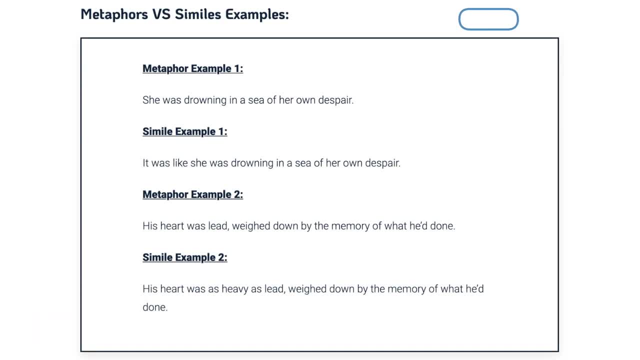 compared by replacing the word. So an example of a metaphor would be: she was drowning in a sea of her own despair, Whereas a simile is kind of more of a direct comparison. by using like or as, So kind of giving the same example, it would read something more like it's as if she was drowning. 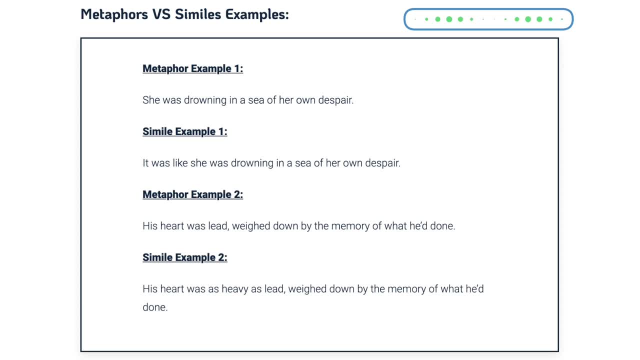 in a sea of her own despair. One more example of a metaphor is saying his heart was lead, weighed down by the memory of what he had done, Whereas if you use a simile, it would say his heart was like lead, weighed down by the memory of what he had. 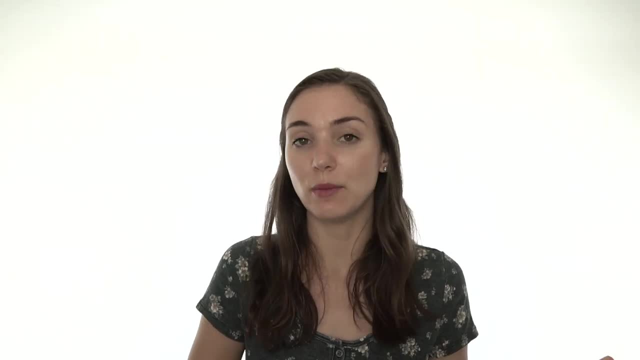 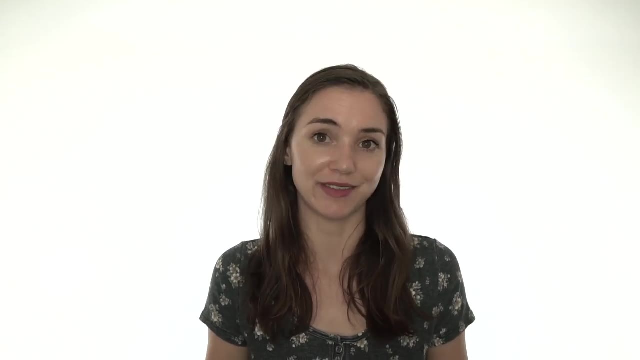 done. Now there's kind of instances where you can use one or the other. I personally like metaphors a little bit better because it brings you closer to the character, it's more impactful, But there are places for both and you just have to know the difference. Literary device number 13 is: 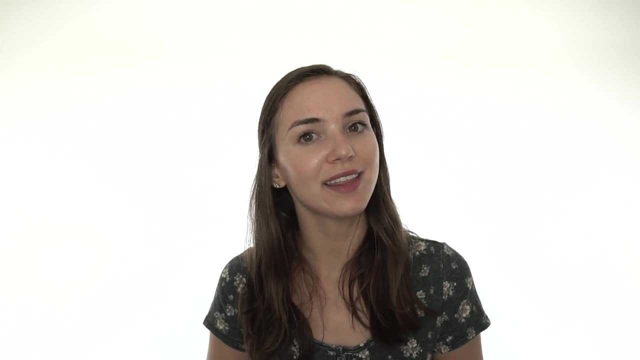 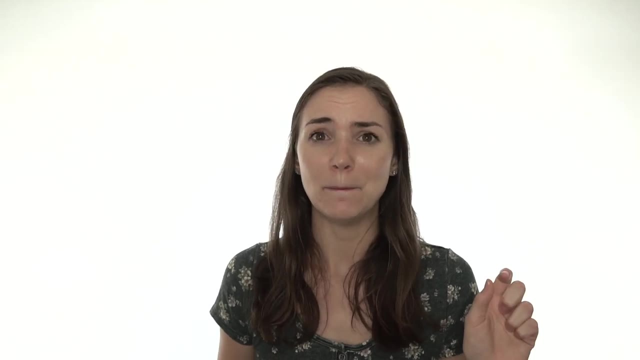 onomatopoeia, And for those of you who can't spell it, I am right there with you, But essentially, an onomatopoeia is a word that's used to describe a sound, And so something like bang or snap. 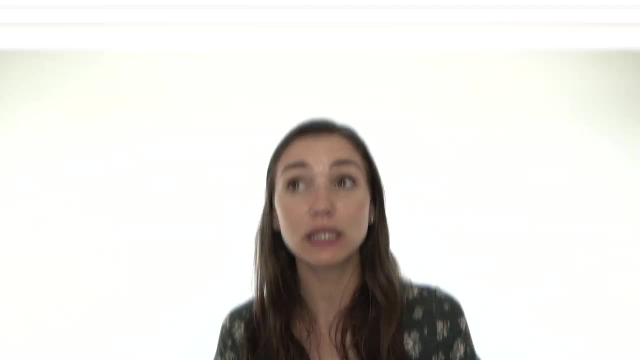 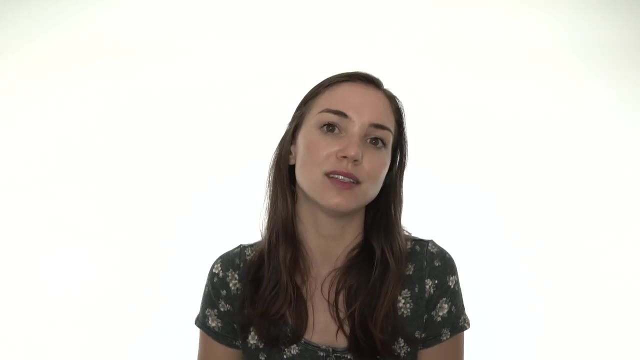 or zip or buzz. all of those are onomatopoeias And typically they're italicized when in writing, just so people know that this is representative of a sound, And the reason you would use this is obviously just to create more of an impact for the reader, something more of an experience. 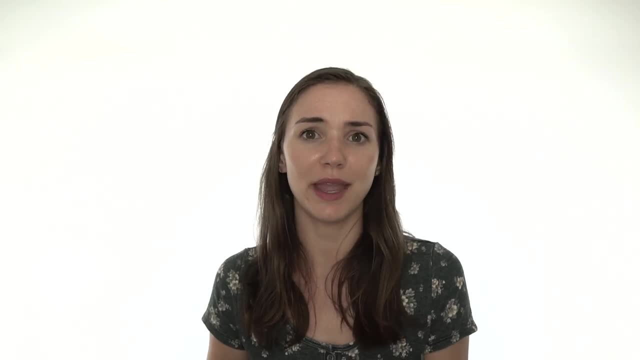 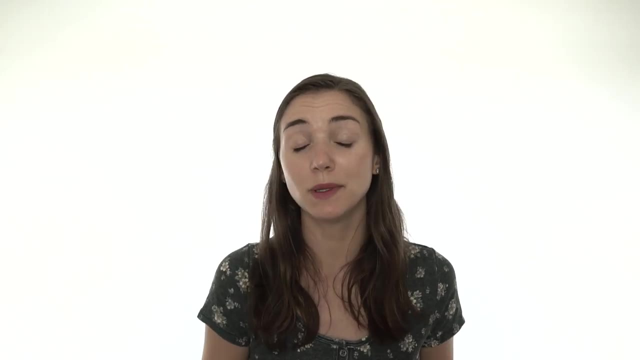 and it hits more of their senses than just saying it made a weird sound. Literary device. number 14: Symbolism. Now, symbolism is used across all literature. It's something that is probably the most digested that, along with themes, when people do decide to kind of pick apart what they've read. 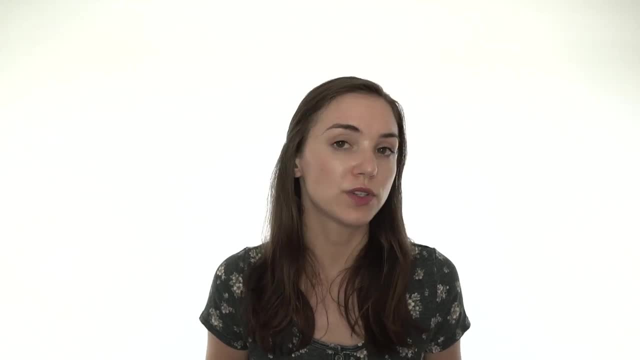 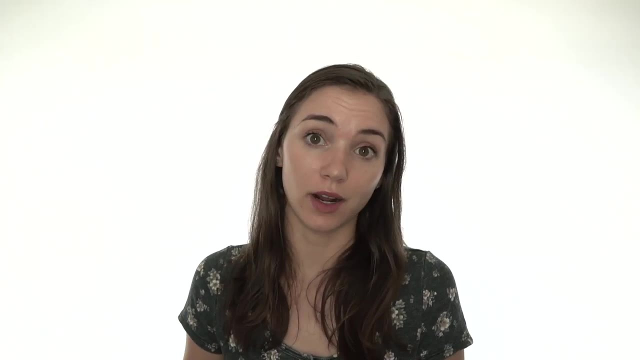 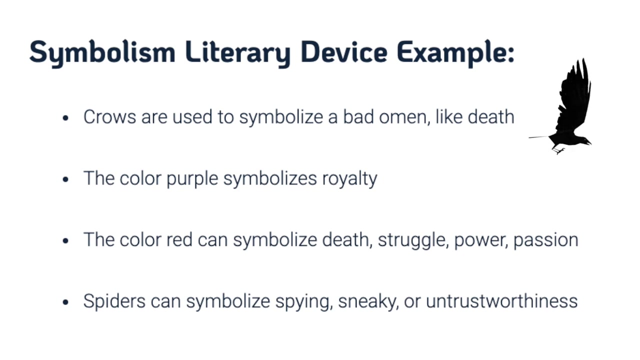 Basically, symbolism is the use of a specific element or situation or something in order to symbolize something more drastic or bigger, And this can be a message, an idea or a concept. So an example of this is crows being used to kind of predict death or tragedy coming, or a storm also. 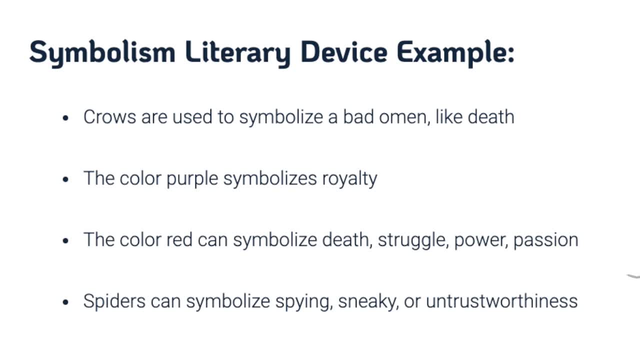 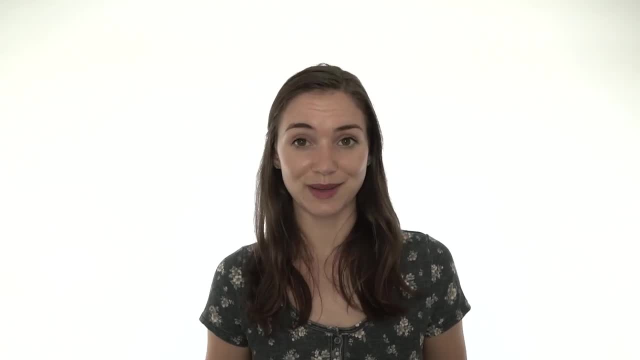 being bad, or the color red predicting violence, or even spiders symbolizing something that's sneaky or not quite right. So there's a lot of different things that you can use here And you can create your own symbolism. If you are writing a story that's in your own world, create something that. 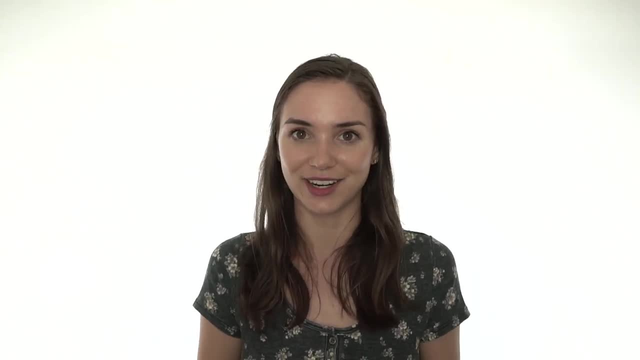 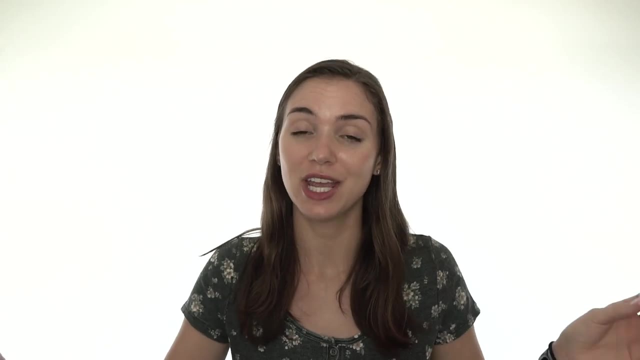 is common knowledge there, like crows are for us here. Literary device number 15 is tone. Now, the tone has the power to completely transform your story from start to finish, And the tone is essentially the narrator's thoughts, feelings or opinions about what's going on And not so. 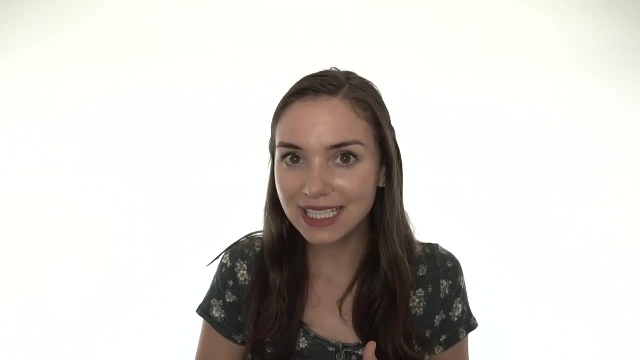 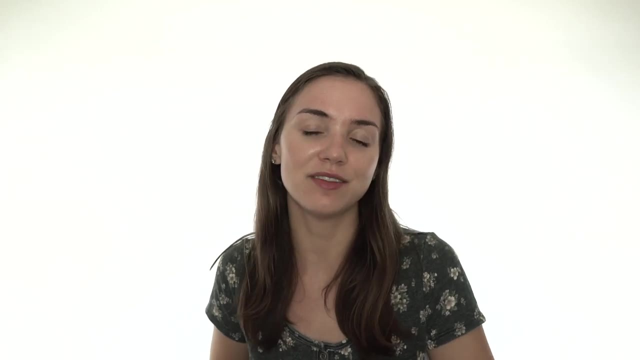 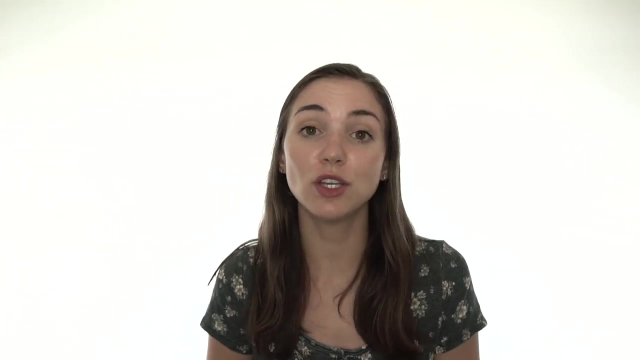 much the actual thoughts, but how what they're saying is written and what that, what perception that leaves for your readers. So can they tell if the narrator is happy or annoyed or sad about what's happening in the story? That is your tone, And so it's something you really want to think. 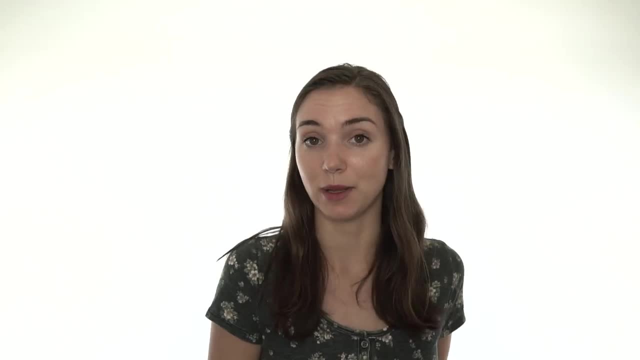 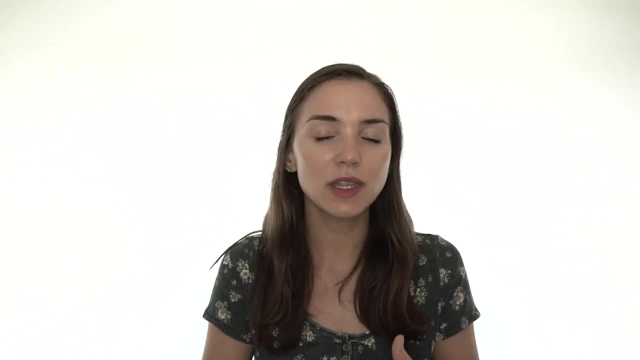 about when you're crafting your story. It does also play into diction quite a bit. So if you're using a formal diction, your tone is probably going to be more straight-laced, uptight, something a little bit more along the way. So if you're using a formal diction, your tone is probably going to